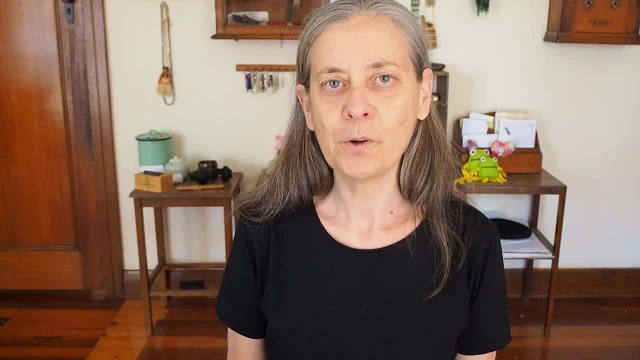 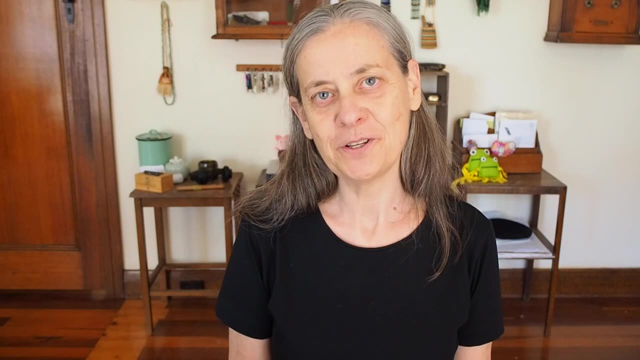 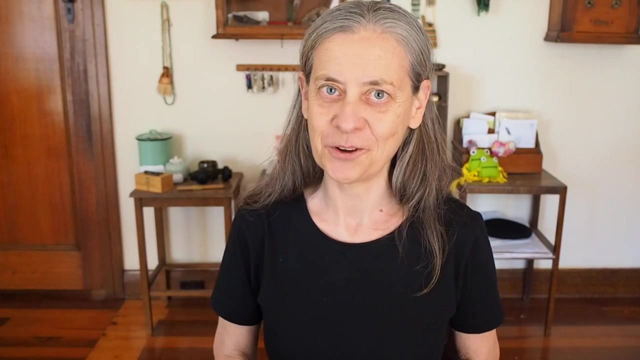 Hi, One of the most common questions I'm asked when teaching kids to sew is: what needle should I use? So today I'm hopefully going to dispel the myth that little kids need big, thick, fat and blunt needles to sew with. So let's begin. Okay, oops, sorry, I forgot to tell you. 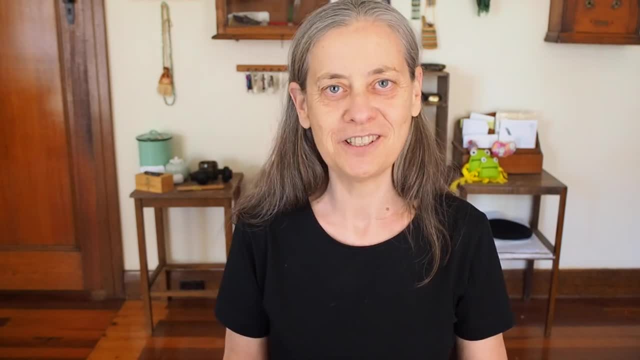 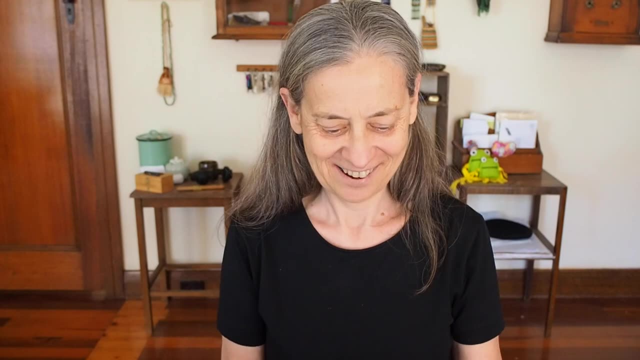 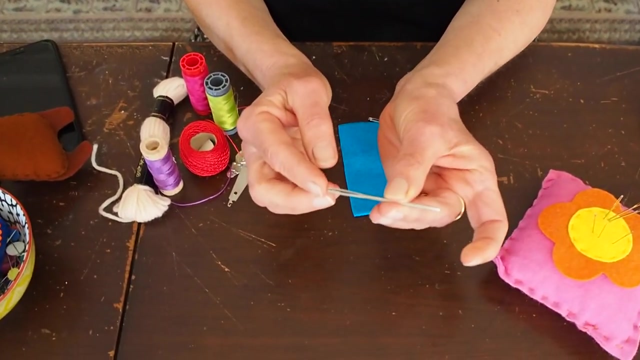 my name is Trixie Simons and you can find me over at SewASoftycom where I give you tips, tricks and projects to help you sew with your kids. Now we can get started. Okay, so this here is a thick, blunt fat needle. It's got a nice big eye, but often parents think that 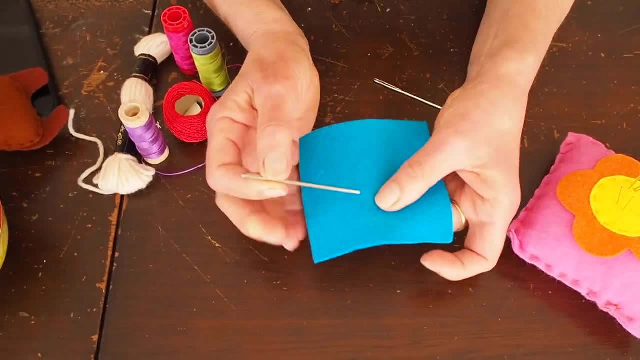 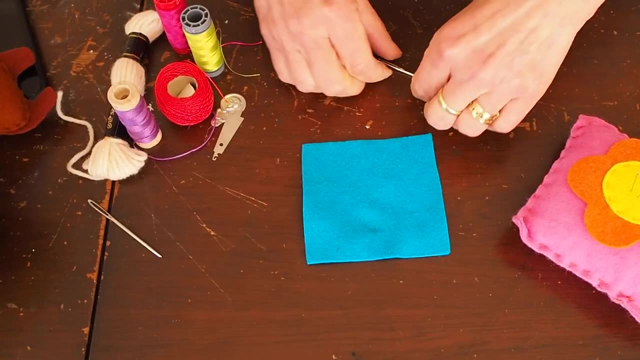 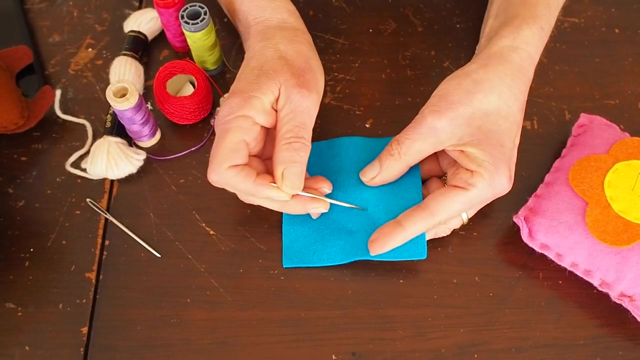 this is a great needle to sew with their kids. Let's see if I try to sew with this. it doesn't work, Okay. our next option would be a thick needle with a sharp point. Let's see how that goes. Okay, you can actually put it through the fabric. 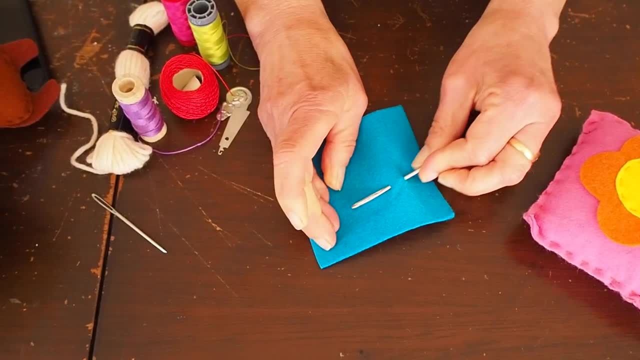 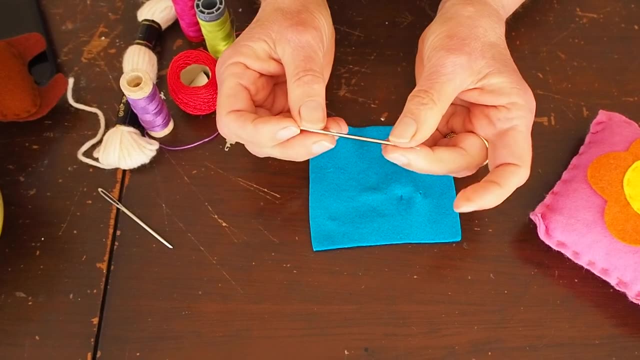 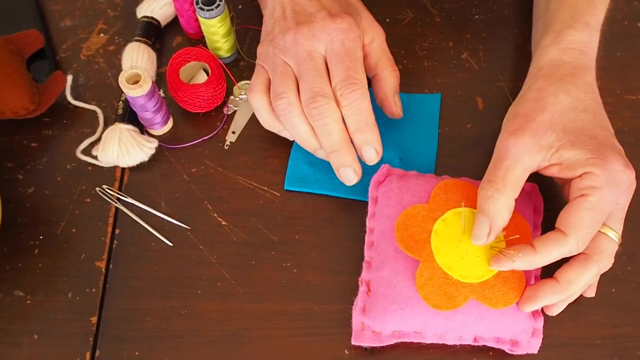 but it's really really, really tough to pull, and if you give your kids one of these needles to sew with, they're probably not going to enjoy this sewing experience. So let me show you the sorts of needles that I like to use. So my favourite needles are what are called chenille. 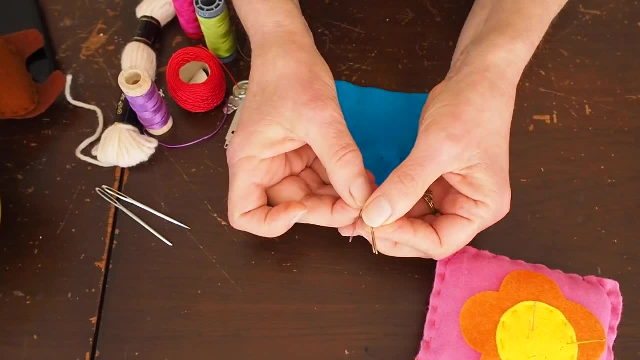 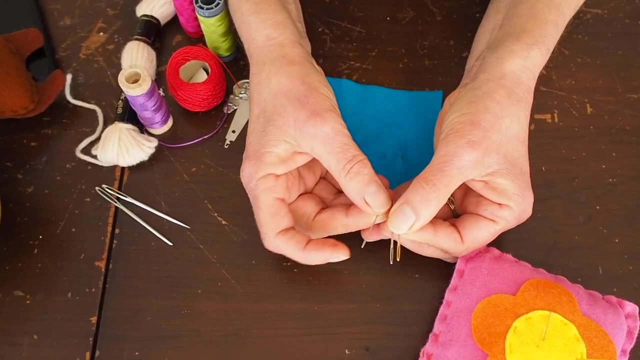 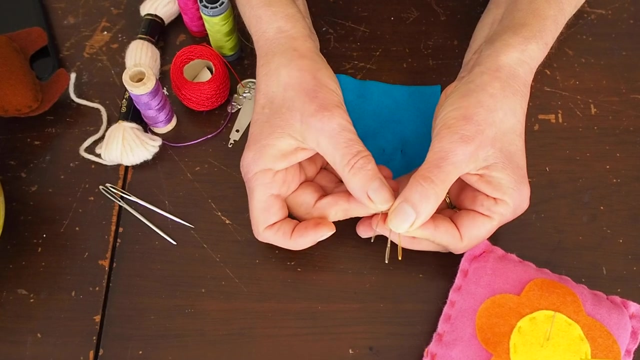 now chenille needles come. I hope you can see in different sizes. These are only some of the size. there are actually lots more. I like to use the smallest chenille needle I can find, but you can only use the small chenille needle- the smallest, if you're using a very thin cotton. 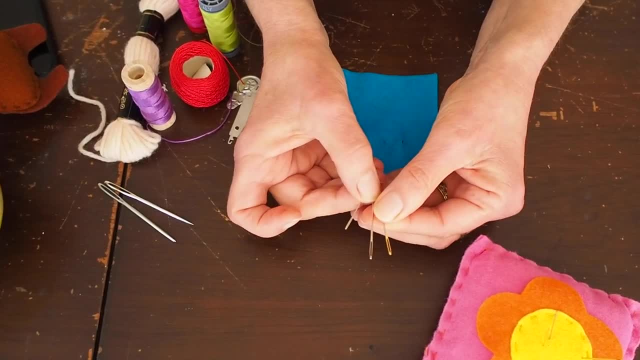 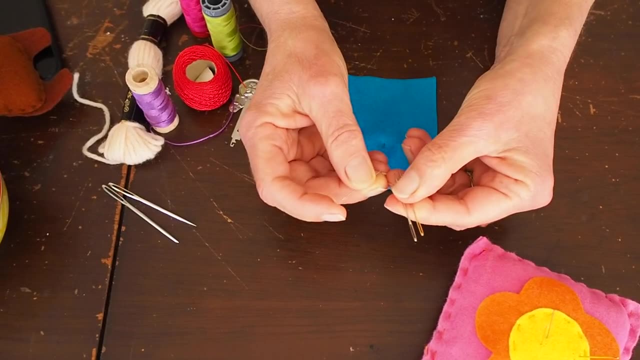 If you're using something like a wool or an embroidery thread, you're going to need to use a larger chenille needle which has a larger chenille needle, which has a larger chenille needle which has a larger hole. So let's just have a quick look at the different sorts of- oh, actually, 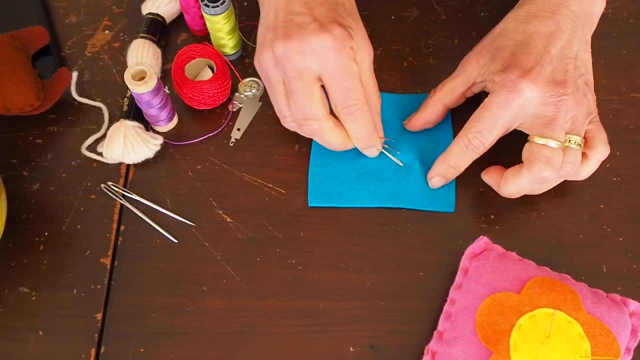 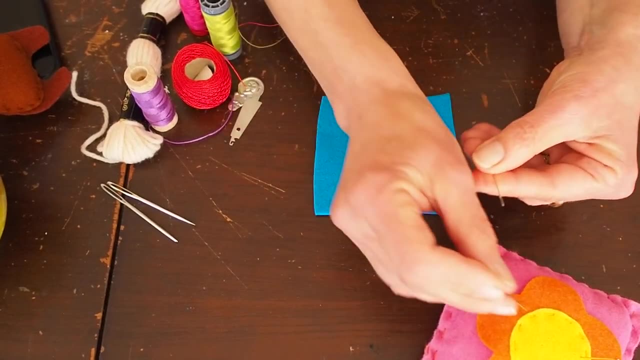 I forgot to say you don't have to just use chenille needles. I'll put these down for the moment. You can use ordinary sewing needles, but they do have a very, very small eye, or an embroidery needle, which does have a larger eye, but it's still not as large as the chenille needles. 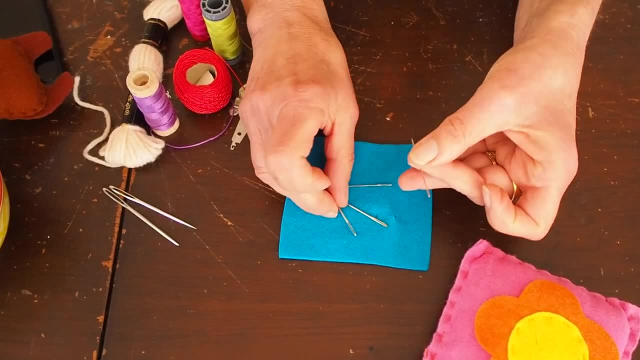 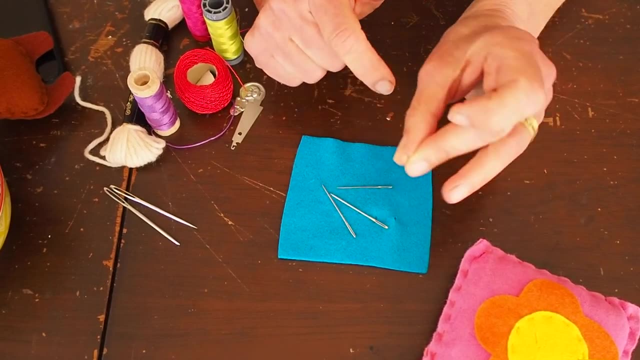 So what I'm saying is, if you don't have a chenille needle at home and you really want to sew, any sewing needle will work. as long as it's, you can thread it and it's got a nice sharp point and it's not too thick. 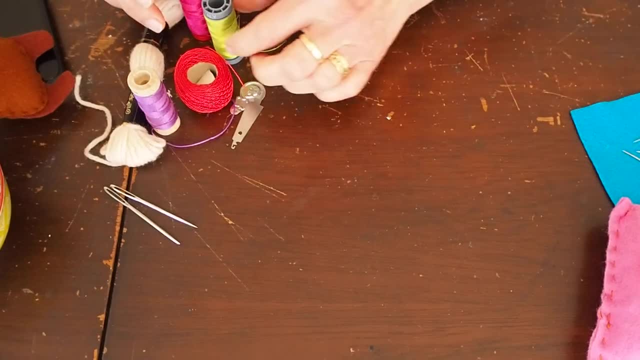 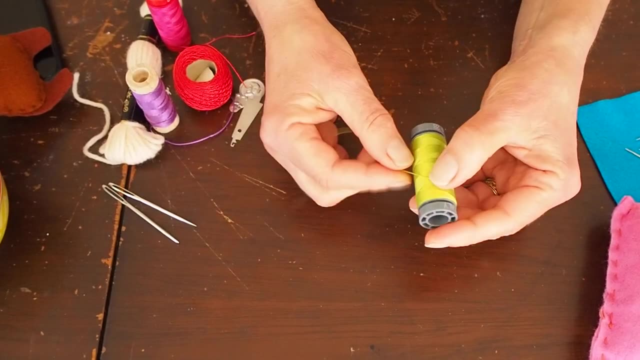 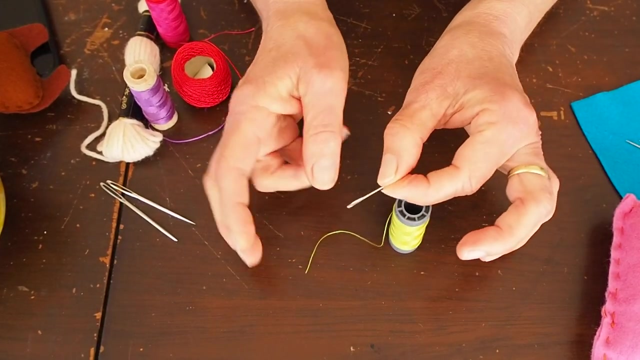 So let's go over here. I'm going to show you some of the different threads that you can use. My favorite is: I just love using ordinary sewing cotton. It's nice and thin, it's easy to sew and you can use a really tiny chenille needle to sew with. And actually I did forget to show. 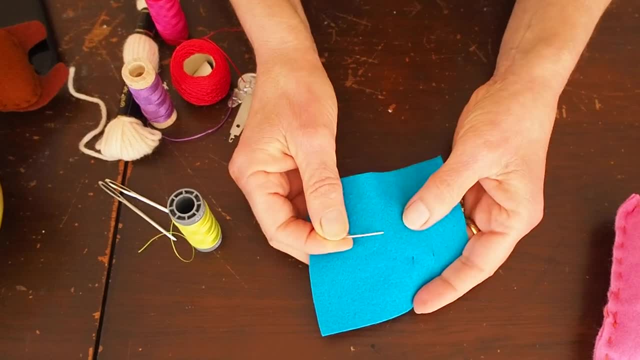 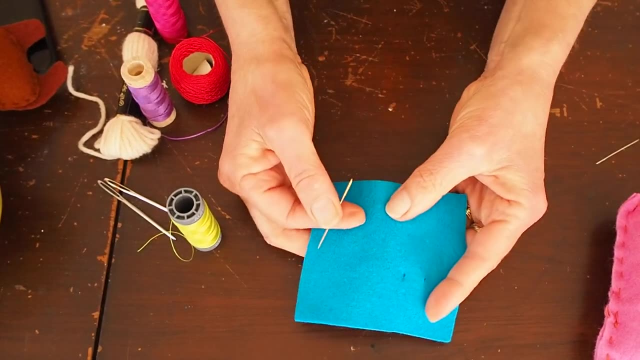 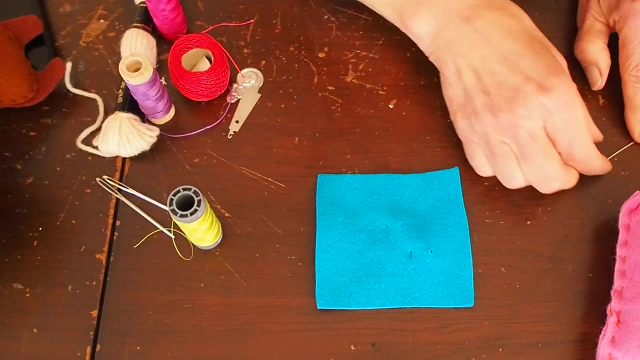 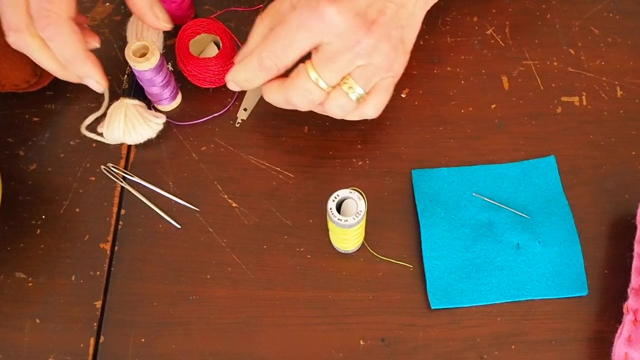 you how easy it is to show to sew with these needles. Look, it just goes in, It goes in out. really easy to pull through. even the slightly larger chenille needles like this one in out. push Back to the thread. So we've got the cotton, which I really like. Then some people like to use 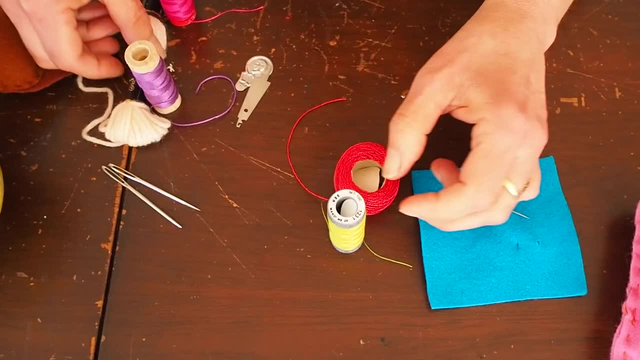 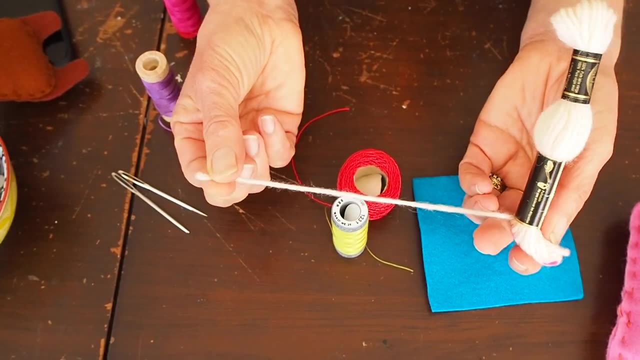 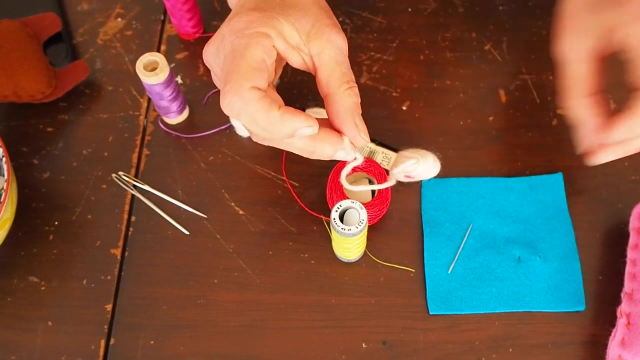 this is a pearl cotton. it's slightly thicker, Or some people actually like to use something a bit like wool with kids. If you're using something thick like this wool, you're not going to be able to thread it through this tiny chenille needle you're going to use. need to use a bigger chenille. 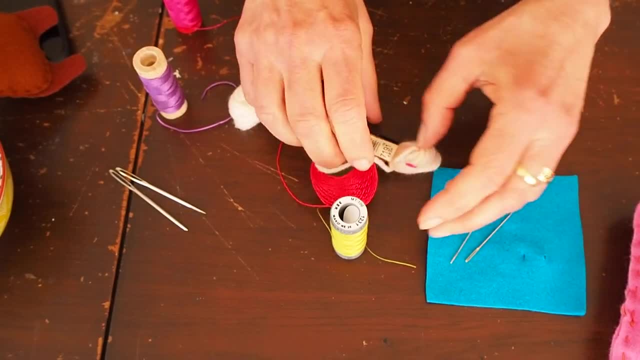 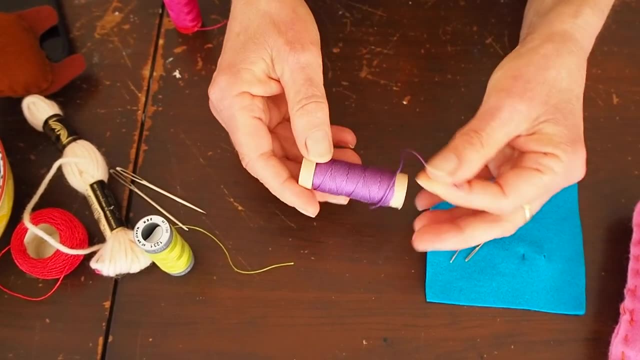 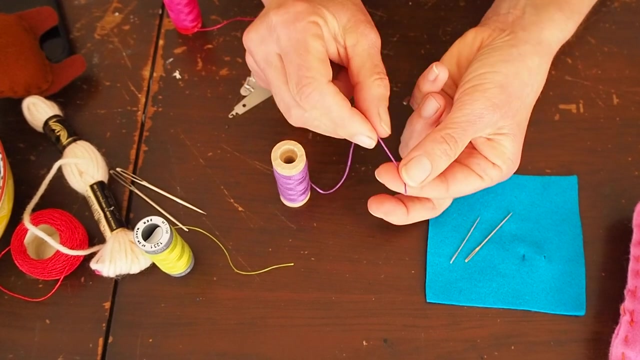 needle like this one, or probably even something a little bit bigger I also like. this is a nice embroidered floss that I like to use. it's an orifal one. it's nice and tightly woven, so it makes. even though it's a thicker thread, it's still quite easy to thread. So let's talk a. 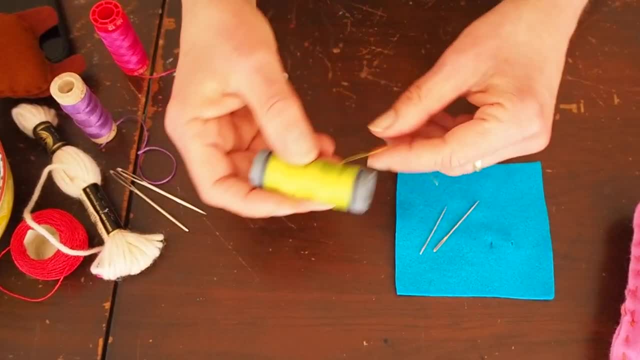 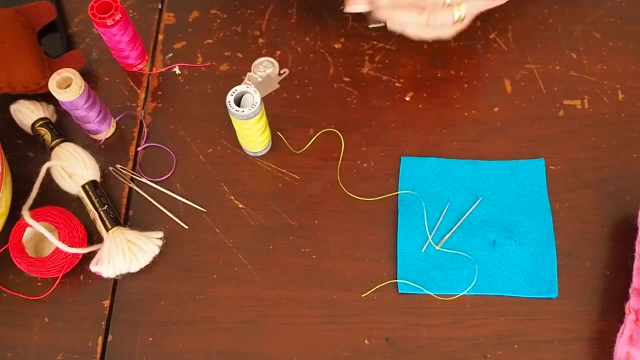 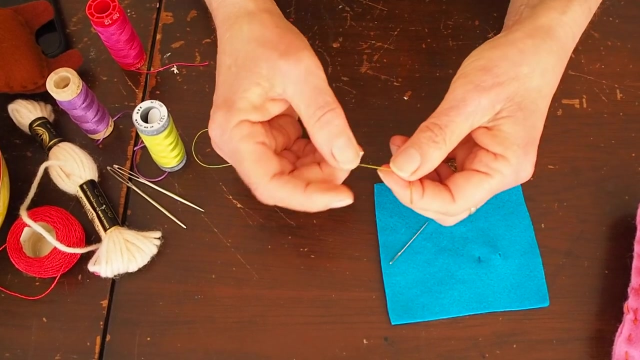 little bit about threading. okay. so one of the reasons I use this cotton- I'll just cut a little piece off- because it's easy to thread and because I can double it over. Now people sometimes ask you know, or get their kids to thread the needle, which is really good. if you've got a big class, you might. 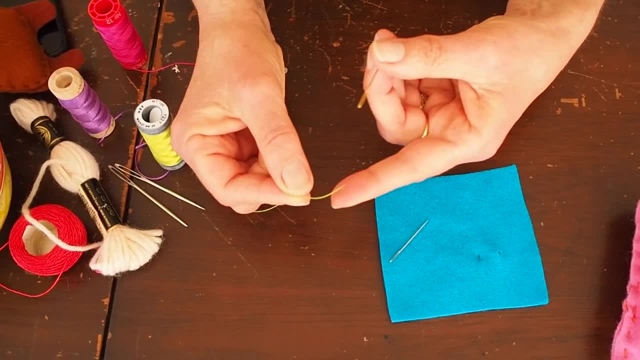 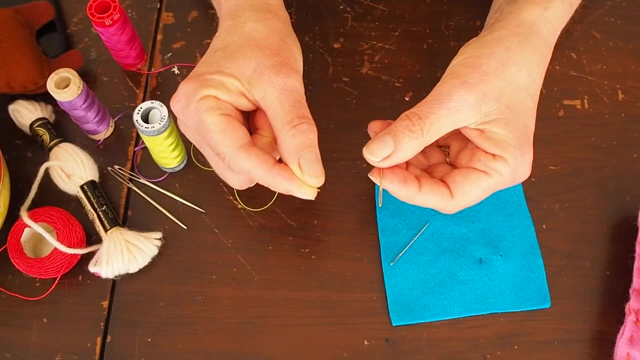 want to get the kids using a needle thread, and I'll show you how to do that. So I'm going to show you how to do that in a moment. but when you're getting your kids to thread, you don't need a long bit of thread. you need a short piece of thread, just the tiny little bit that kids hold. 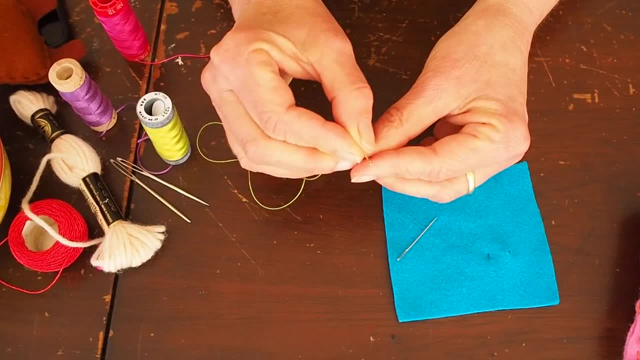 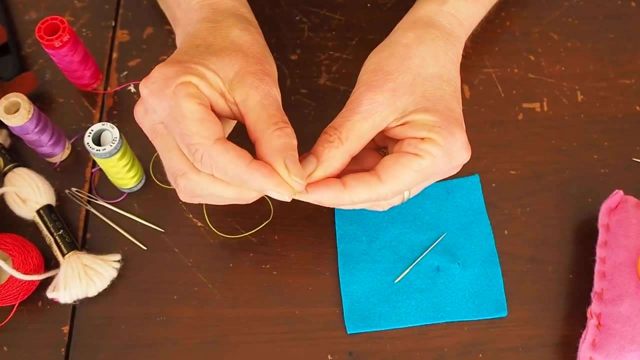 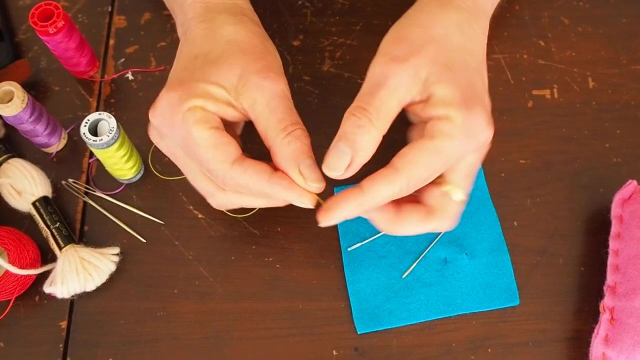 between their thumb and forefinger, and then it really makes it quite easy to thread. I'll just do it in this here one. here it's a smaller needle- just the tip of your thread and carefully and it goes through. Now, sometimes if the ends of your thread is a bit full and you don't have enough, 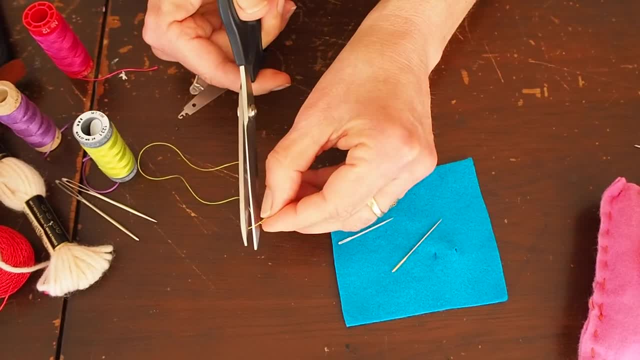 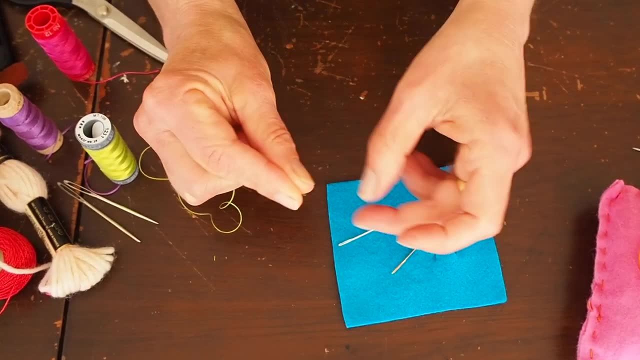 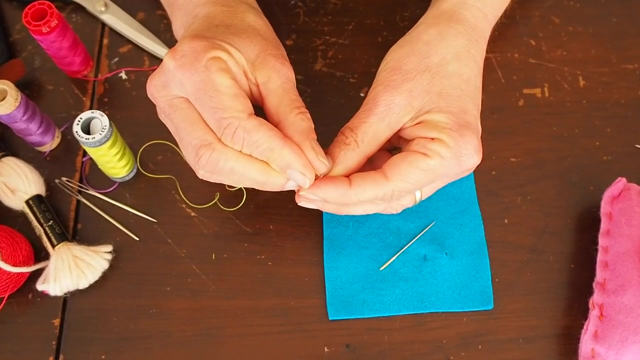 thread, it's a good idea just to cut it. that sometimes helps. There is the old lick and pinch method, but probably these days most people don't want to use that one. but just a tiny bit of thread through your needle and there we go and, like I said, what I do like about usually ordinary 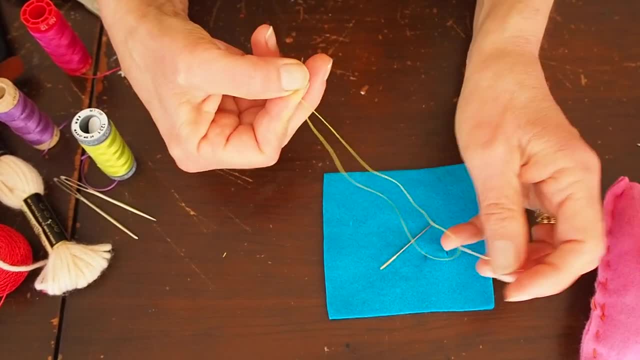 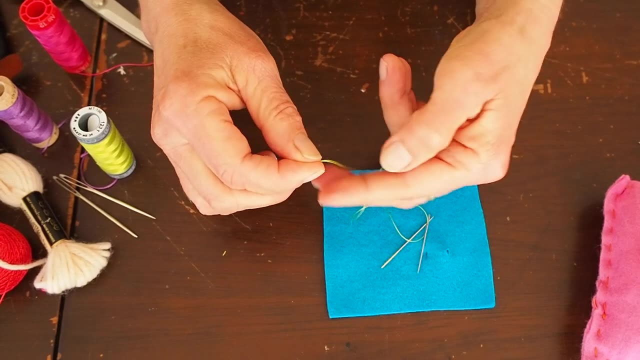 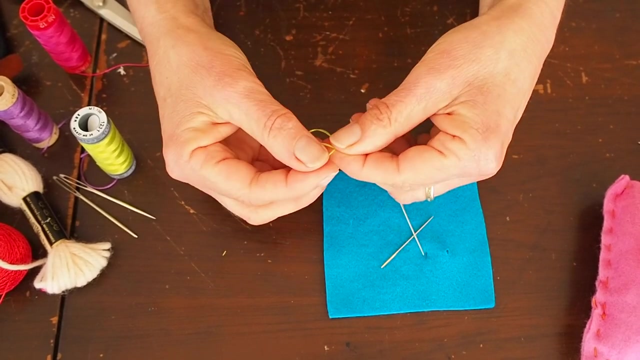 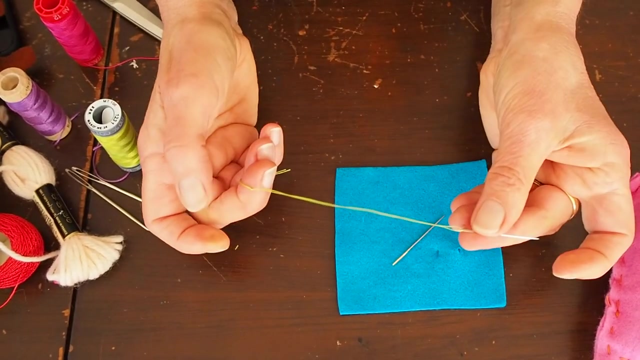 sewing cotton is. I always get the kids to bring the two ends of the thread together and knot it, and that's just simply by twirling the cotton, the thread, over their fingers, taking the loop off and going under and over. and the reason I do that is it is so that the needle 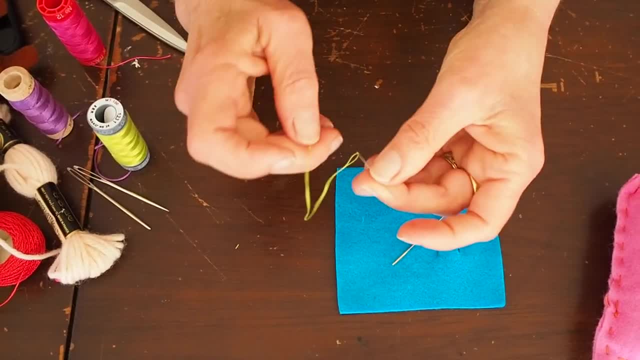 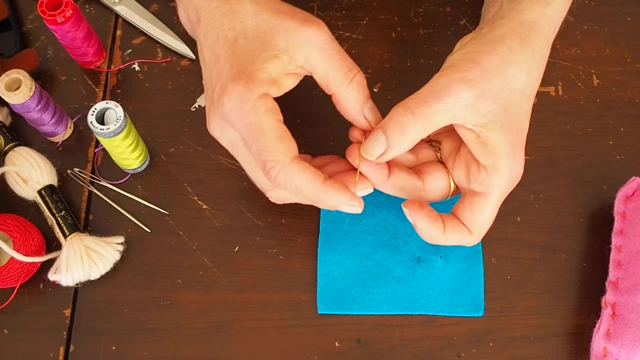 doesn't pull off the thread while the kids are sewing. Now, if you're working with a large group of kids and you don't want kids being frustrated by not being able to thread their needles, and you want them to get their sewing done, so there's two. 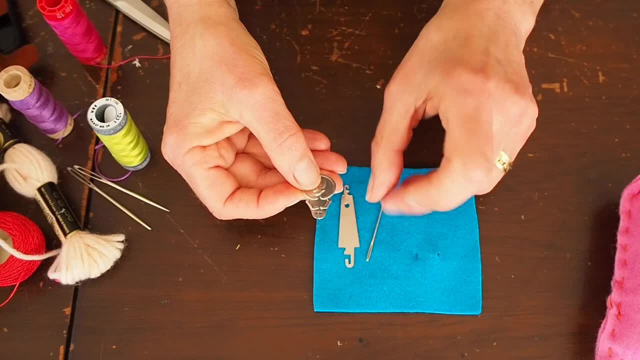 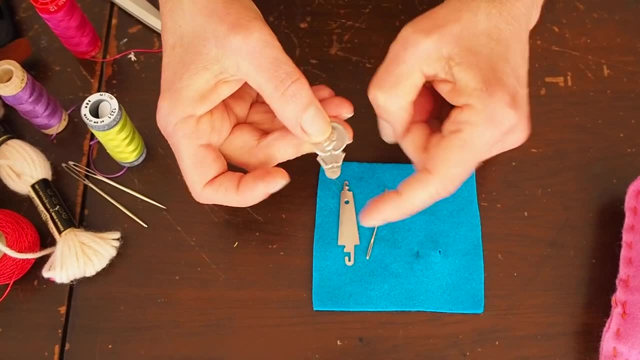 different sorts of needle threaders. This is the old-fashioned needle threader. unfortunately they don't often last very long and they this little bit here- I don't know if you can see it- for breaks off really easy. but I'll show you how to do that. I'll just get a thicker thread here. 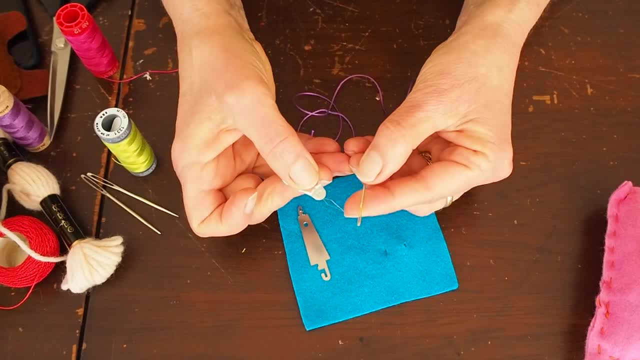 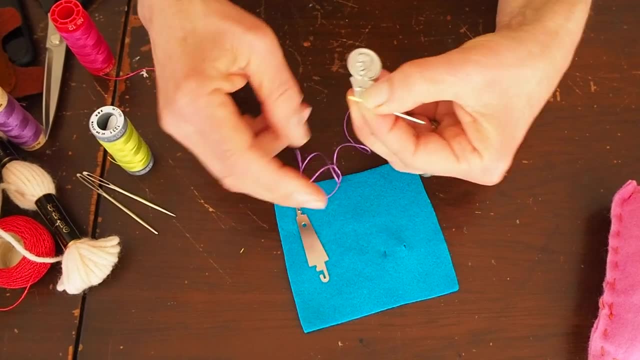 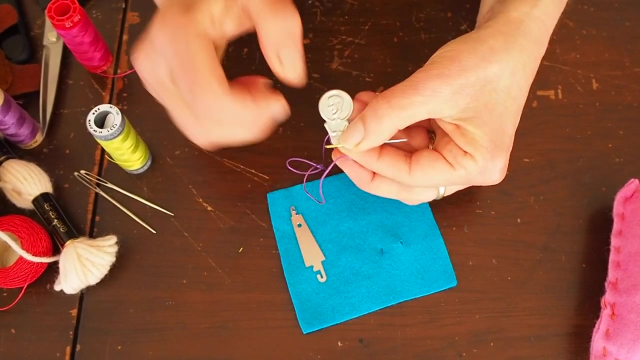 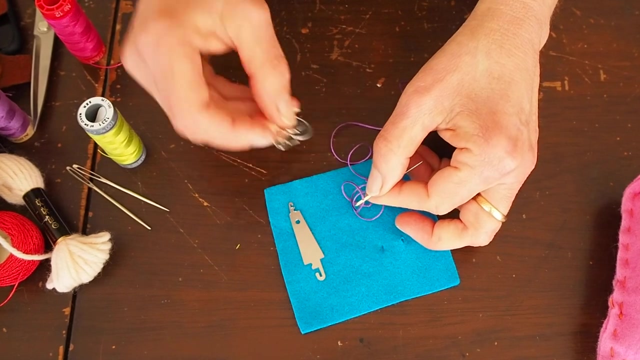 and how you use this one is: you should put this little wire bit of the needle threader through the eye of the needle. you just thread, your push your thread through there and then pull it through and there you go. but of course, like I said, these little bits here fall off pretty easily.